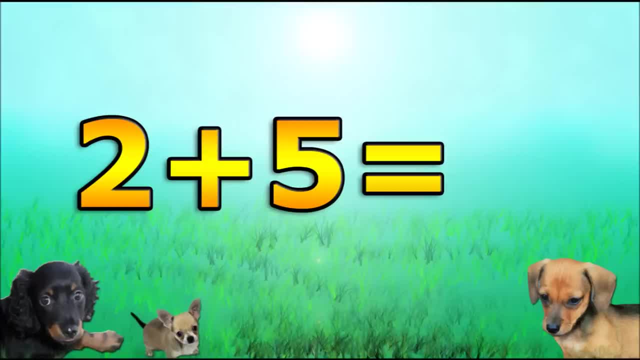 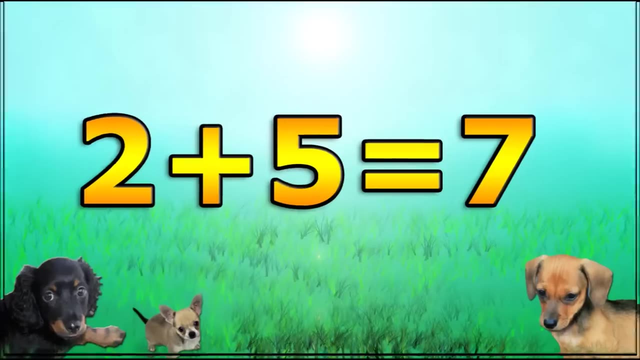 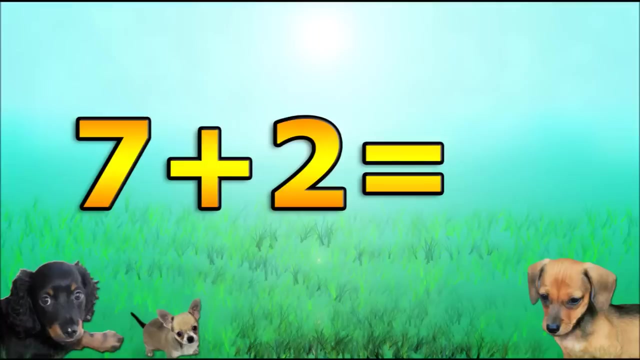 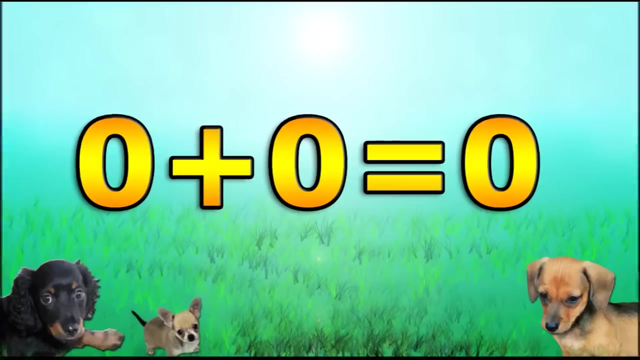 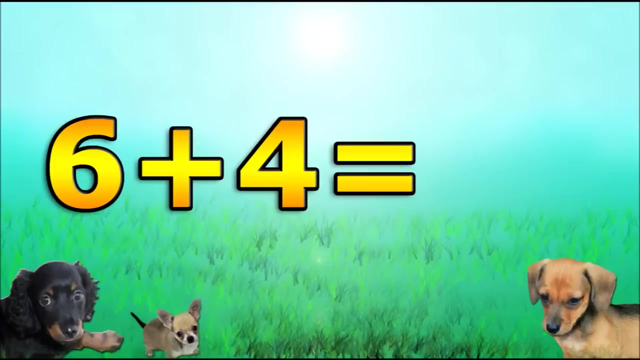 2 plus 5 equals 7.. 7 plus 2 equals 9.. 4 plus 3 equals 7.. 6 plus 0 equals 6.. 0 plus 0 equals 0.. 6 plus 4 equals. 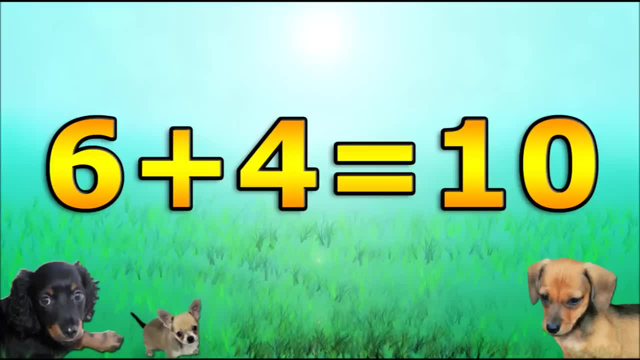 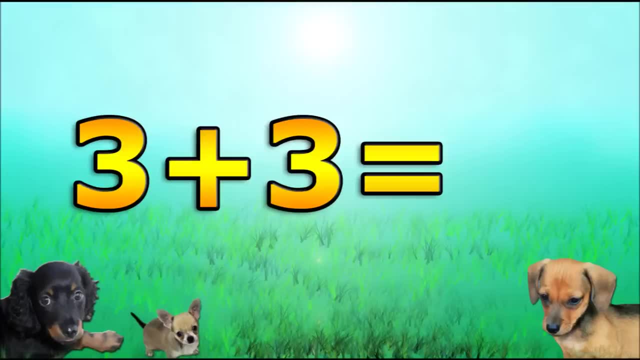 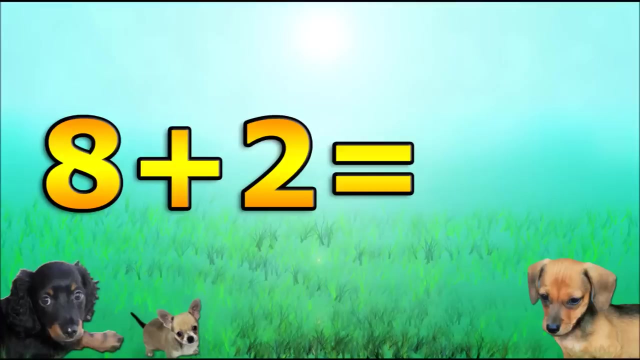 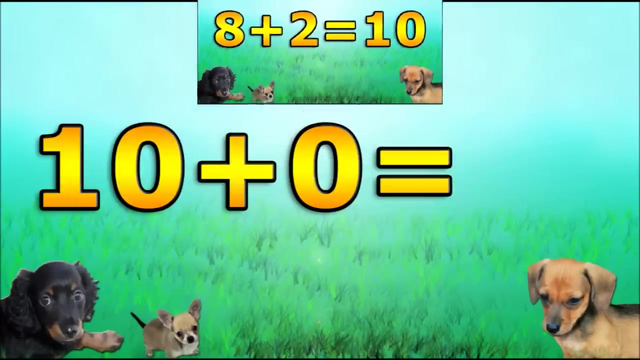 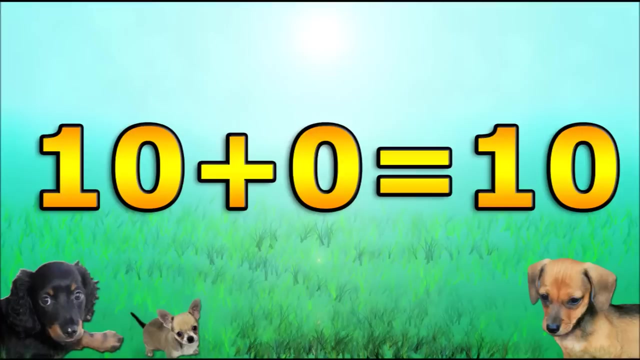 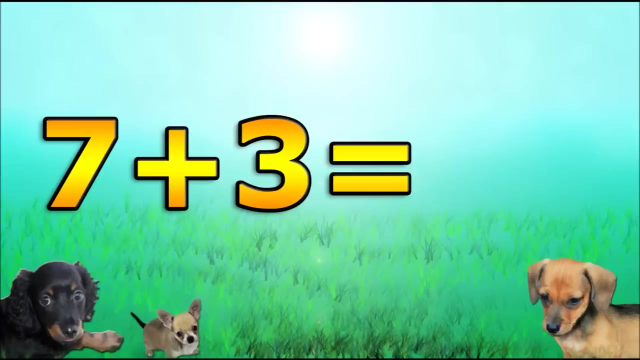 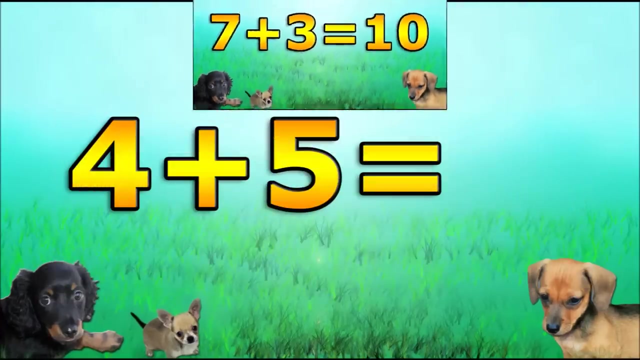 0.. 3 plus 3 equals 10.. 6, 2 plus 3 equals 5. 8 plus 2 equals 10. 10 plus 0 equals 10. 7 plus 3 equals 10. 4 plus 5 equals. 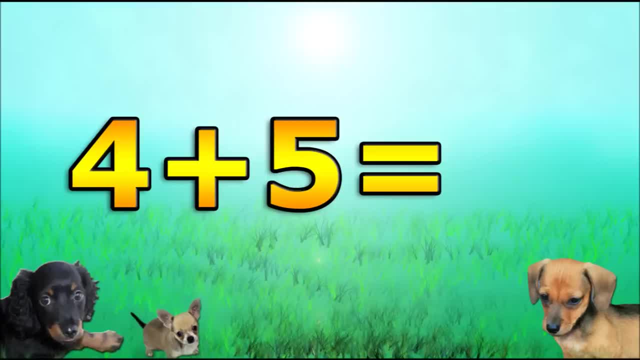 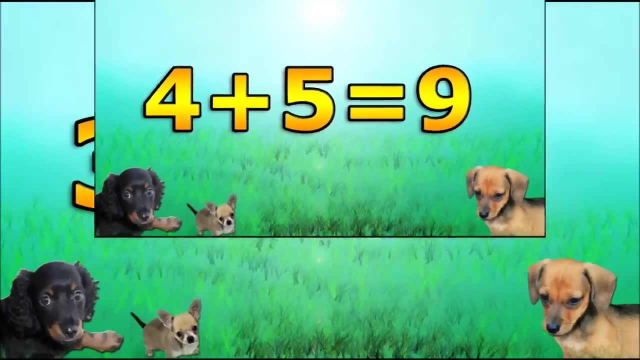 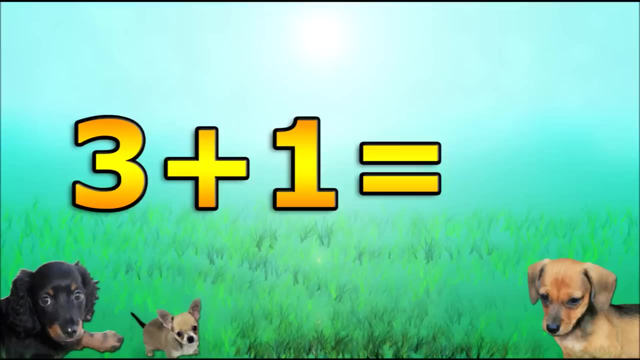 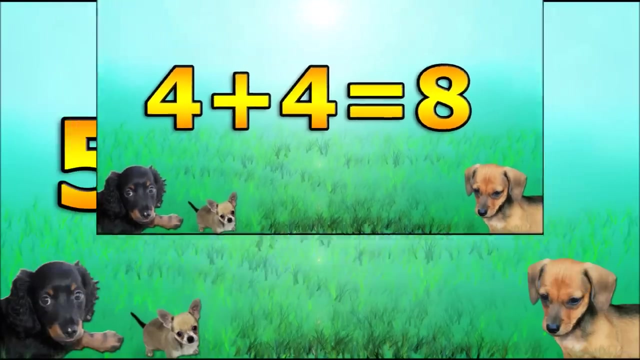 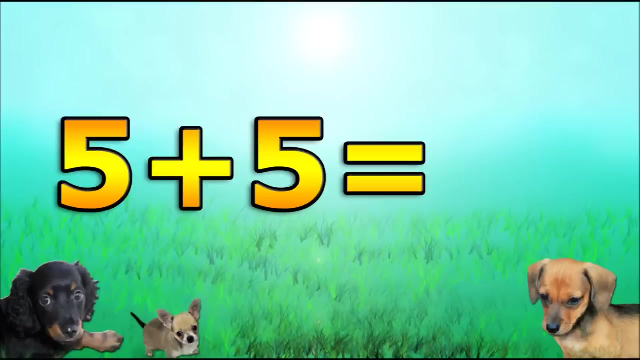 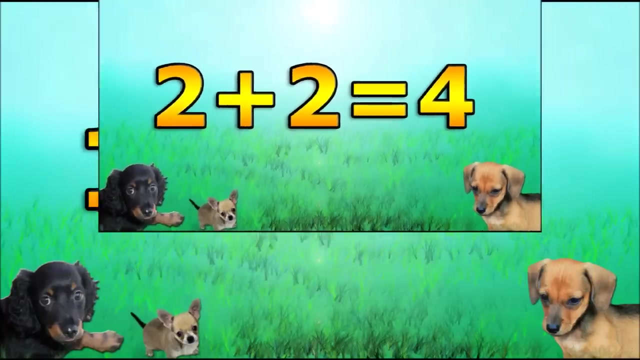 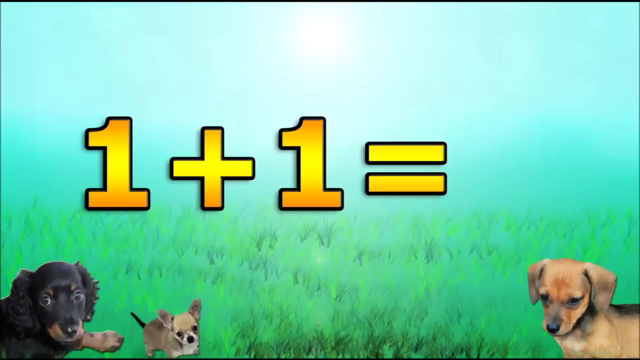 10, 9, 3 plus 1 equals 4. 4 plus 4 equals. 4 plus 4 equals 8. 5 plus 5 equals 10. 2 plus 2 equals 4. 1 plus 1 equals 2. 2 plus a equals. 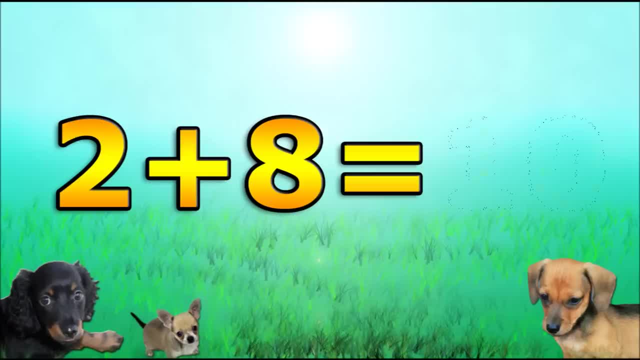 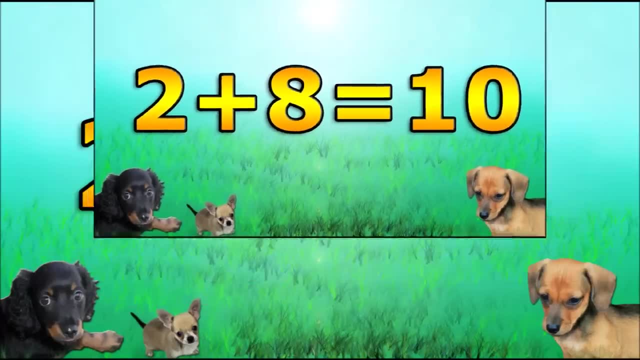 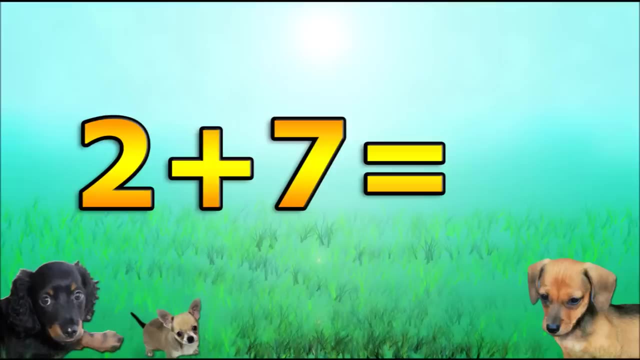 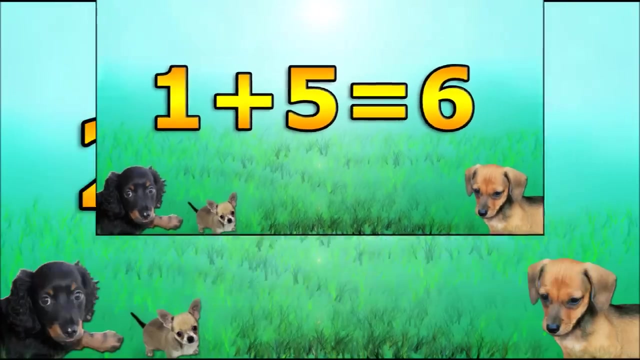 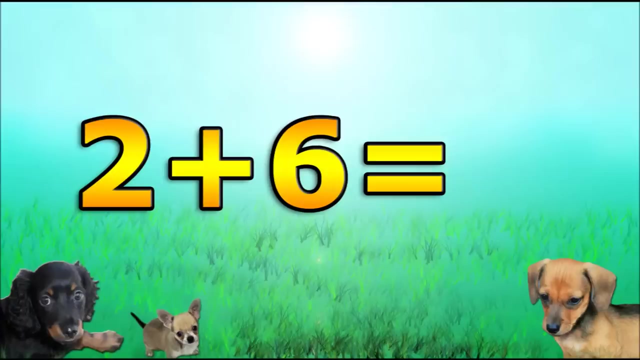 10, 2 plus 7 equals 9, 1 plus 5 equals 10, 2 plus 7 equals 6, 2 plus 6 equals 8, 2 plus 7 equals 9, 2 plus 7: equals 4 plus 2: equals. 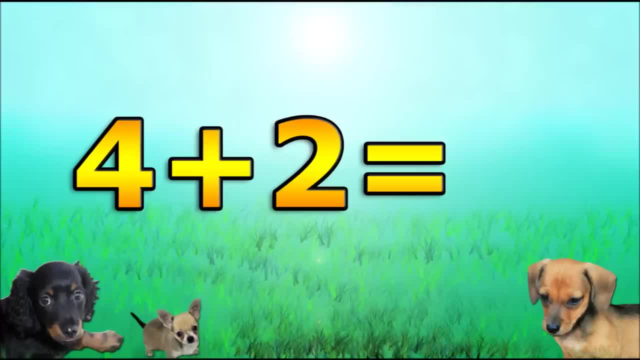 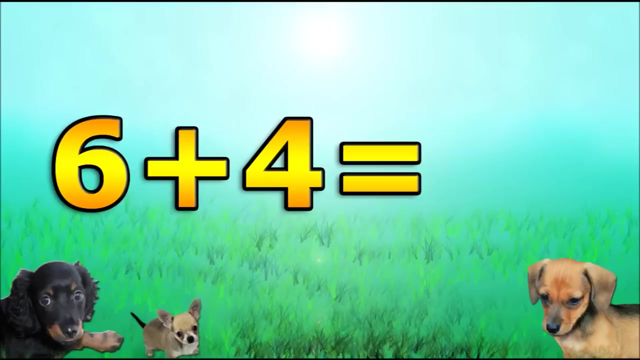 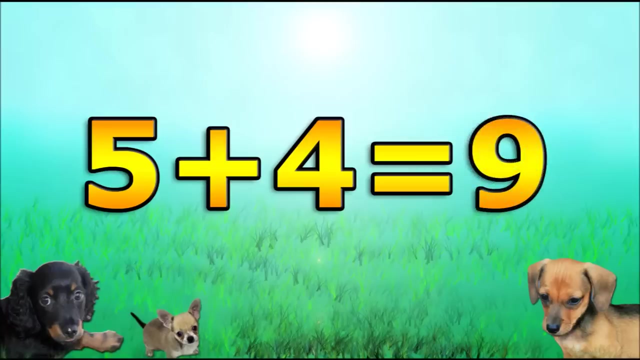 6, 6 plus 4 equals 10. 5 plus 4 equals 9. 0 plus 0 equals 3 plus 4 equals 2 plus 5 equals 5 plus 6, equals 2 plus 6 is equal to 6 plus 7 equals. 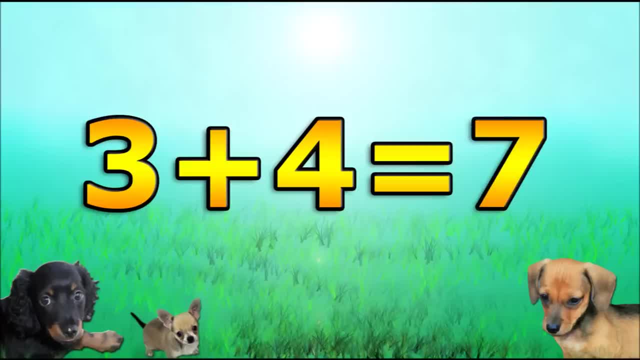 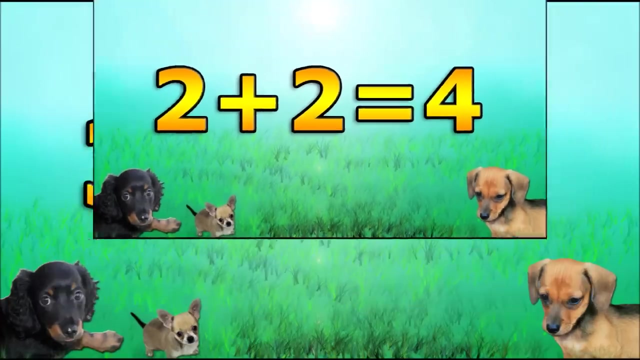 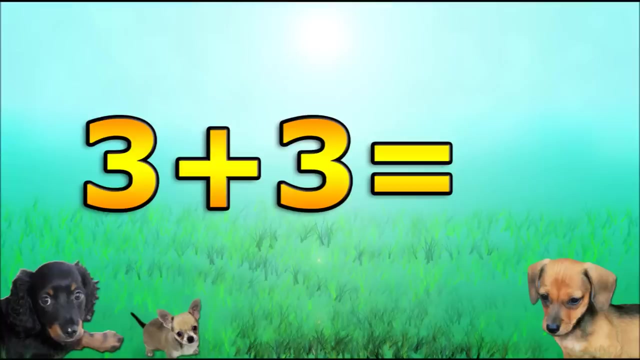 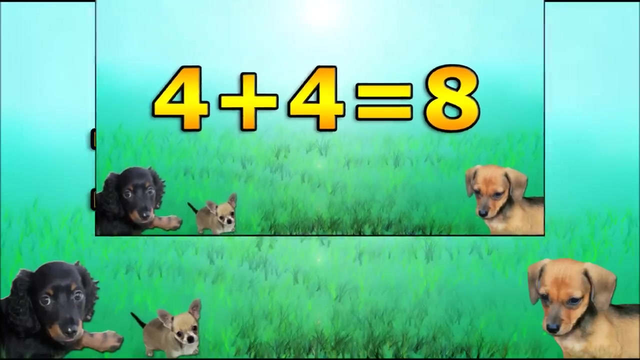 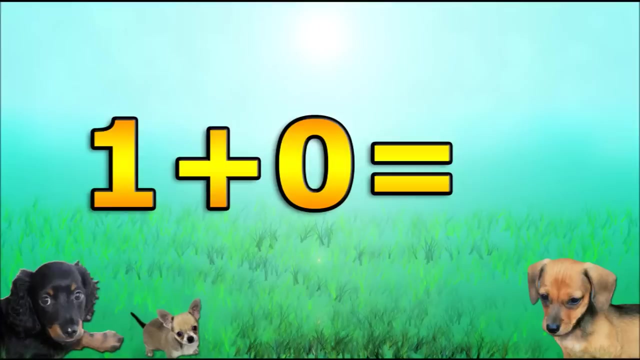 3 plus 4 equals 0. 3 plus 4 equals Two plus two equals four. Three plus three equals six. Four plus four equals eight Eight. One plus zero equals one. Four plus five equals seven, Seven Seven Seven.